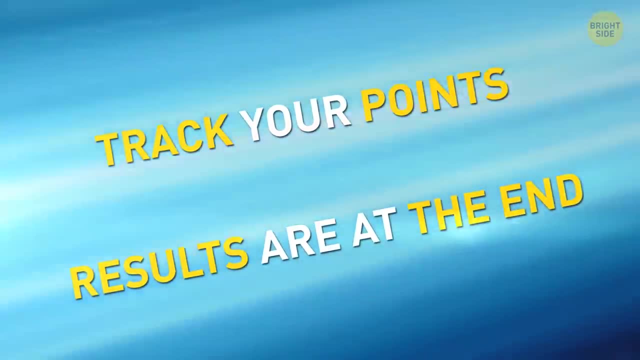 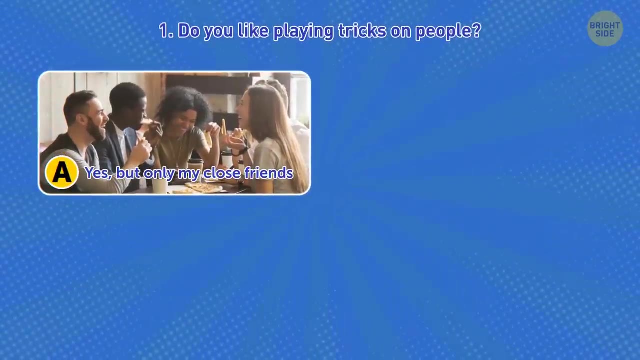 Keep track of your points and check your results at the end of the test. Do you like playing tricks on people? A- Yes, but only my close friends. They know I don't mean it. B- Everyone all the time. C- Never. I'm afraid to hurt their feelings. 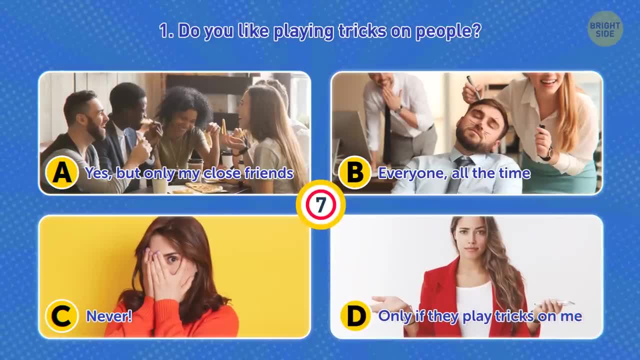 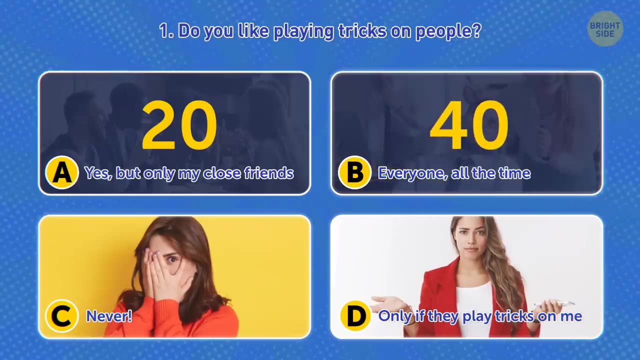 D Only if they play tricks on me. If you picked option A, you just earned 20 points. If you went with B, add 40 points to your basket. Those who chose C earned 10 points. D is worth 30 points. 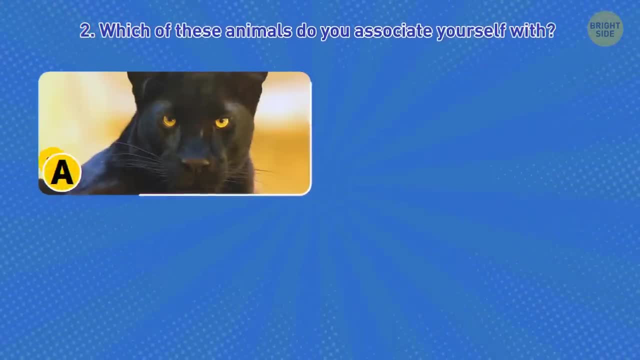 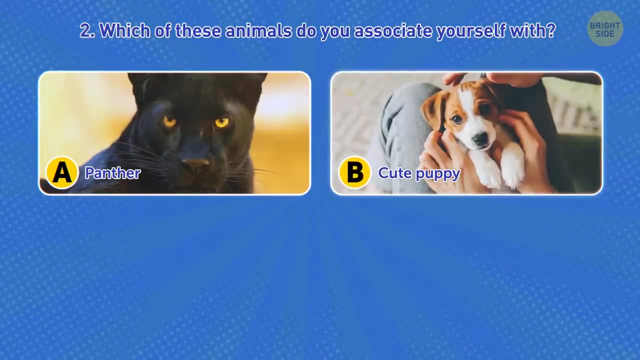 Which of these animals do you associate yourself with? A- Panther- I'm also posh fast and can always protect myself. B- Cute puppy, I wouldn't survive a day without my family. C- Kangaroo: I'm one of a kind and you can't approach me easily. 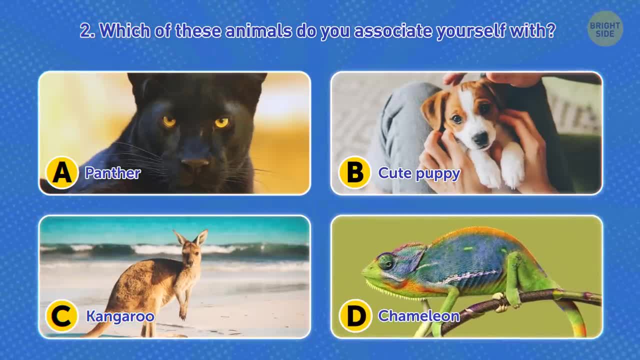 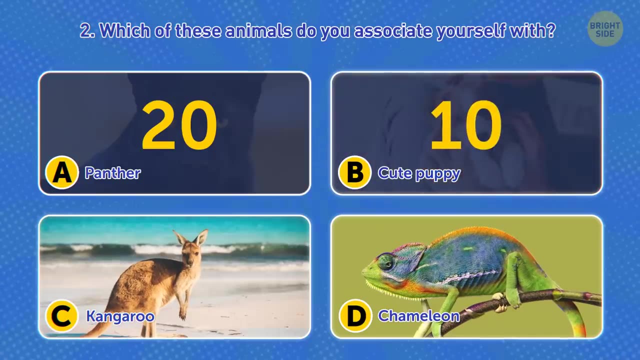 D Chameleon. I can fit into any surroundings. All panthers out there get 20 points. Puppies at heart can add 10 points to their score. Kangaroos scored 30, and chameleons got 40 points. 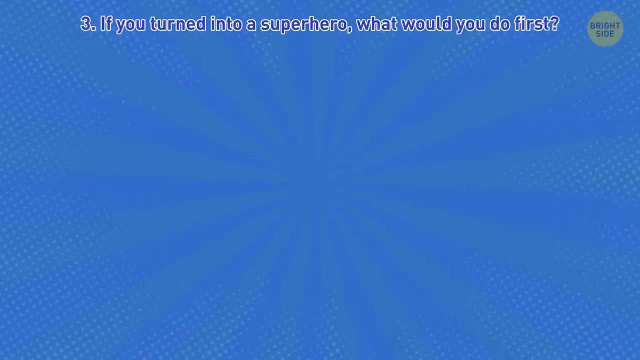 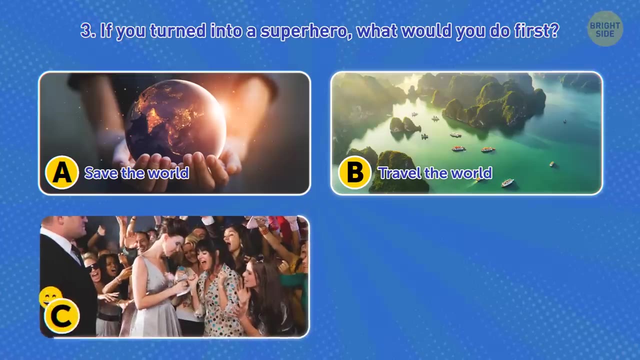 If you turned into a superhero, what would you do first? A. Save the world. B. Travel the world. Being a superhero involves flying right. C. Meet my favorite celebrity. D. Use my superpowers to produce as much money as I've always wanted. 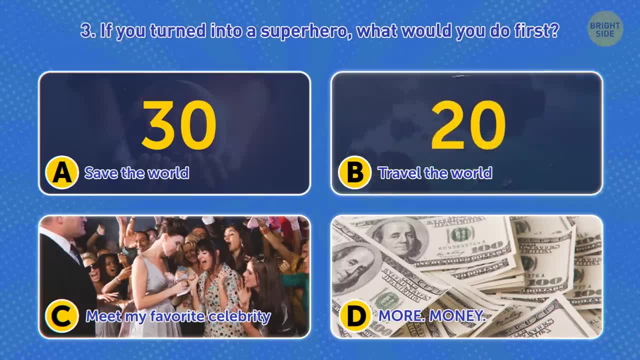 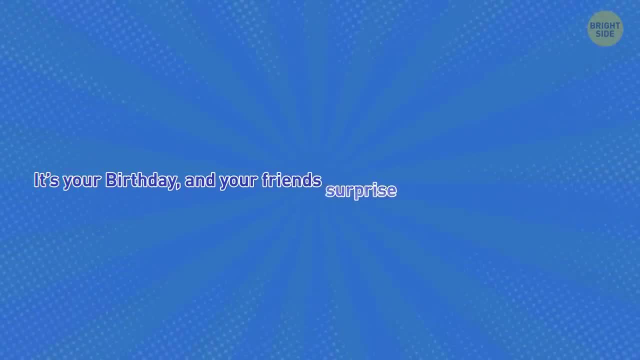 Option A brings you 30 points. B Is worth 20.. C Is worth 10 points. D Gives you 40 points. It's your birthday and your friends surprise you with your dream car. How long will you be happy about it? 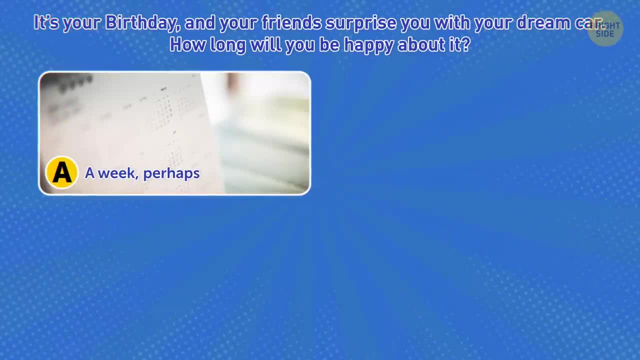 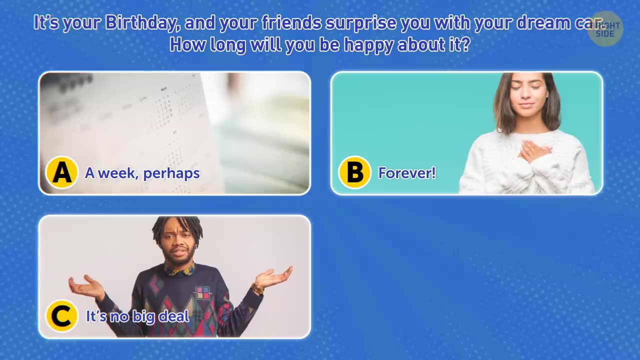 A- A week perhaps, until the joy fades away. B- Forever- It's the gift of a lifetime. C- It's no big deal. It takes way more than that to make me happy. D- I won't accept it. It's too much, and they know it. 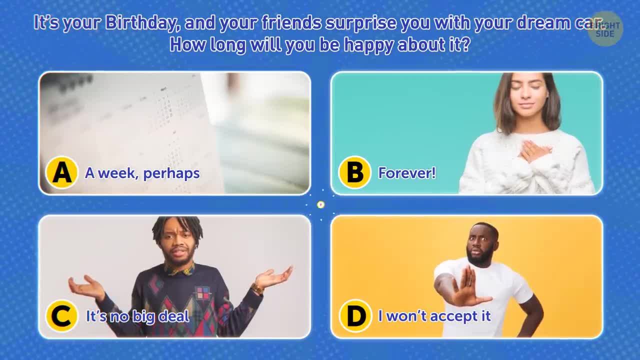 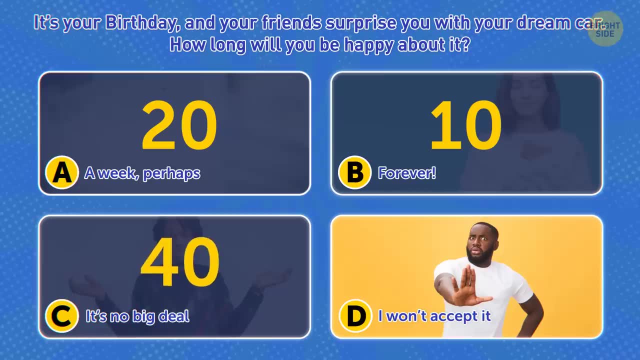 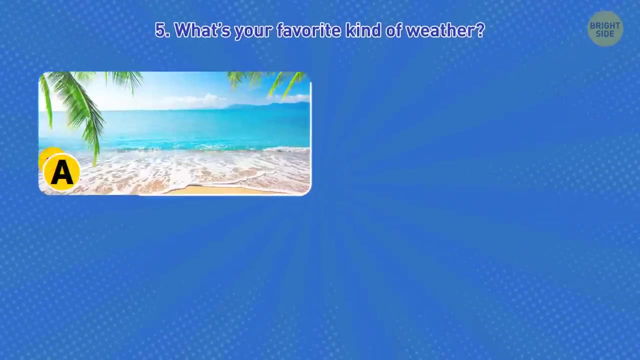 If you picked A, add 20 points to your score. If you went with B, it's worth 10 points. C Brings you 40 points And D 30 points. What's your favorite kind of weather? A, Beach weather, Sunshine, no clouds, heat. 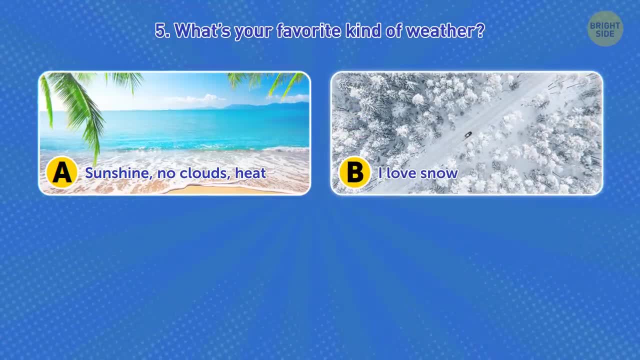 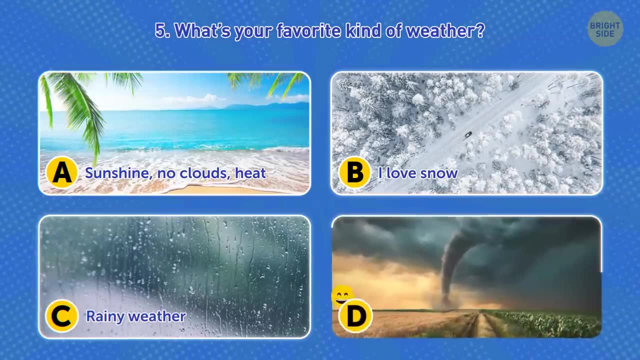 B. I love snow. Playing outside or staying at home on a snowy day makes me happy. C. Rainy weather: D- The sound of it Helps calm me down. D. Extreme weather, Thunderstorms, tornadoes, sandstorms- they make life more interesting. 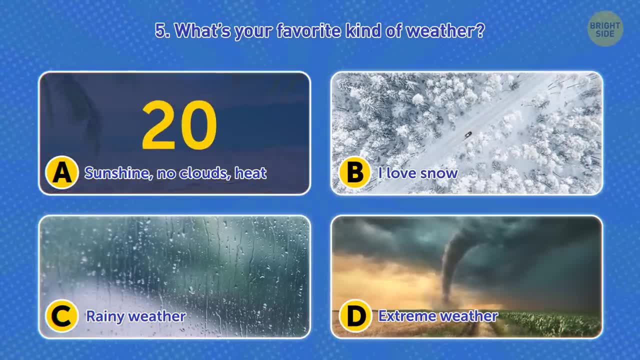 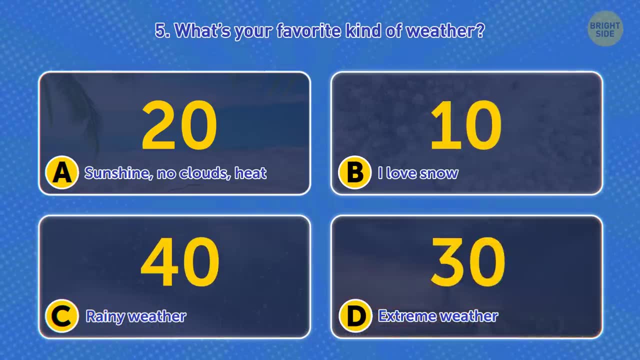 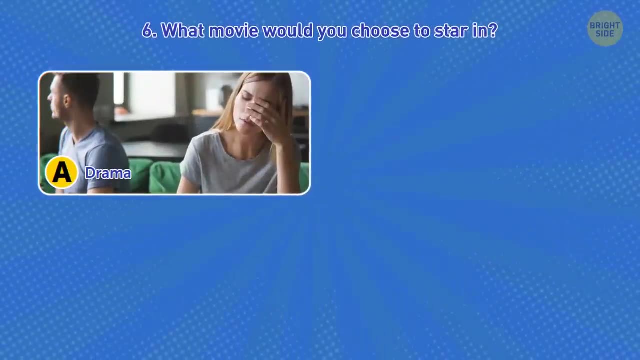 If you prefer sunshine, add 20 points to your basket. Snow fans earn 10 points. Rain fans get 40 points. Those who love extreme weather earn 30 points. What movie would you choose to star in? A Drama. I know how to play it because I live it. 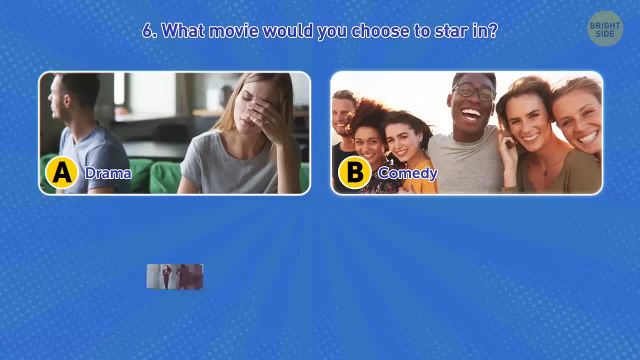 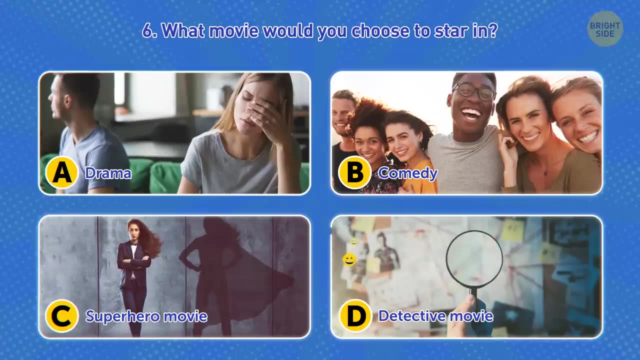 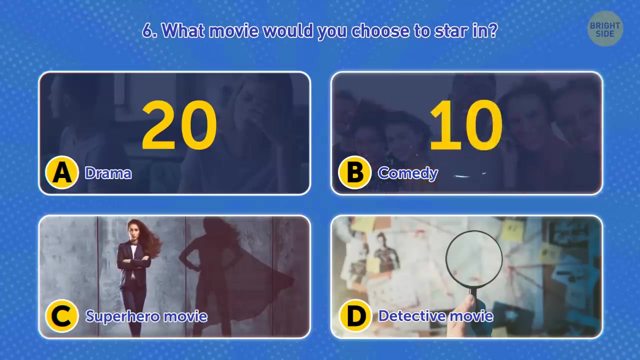 B- My sense of humor and irony will help. C- Superhero movie. I even know what my superhero costume will look like. D- I want to star in a detective movie and solve mysteries. Option A brings you 20 points. B Is worth 10 points. 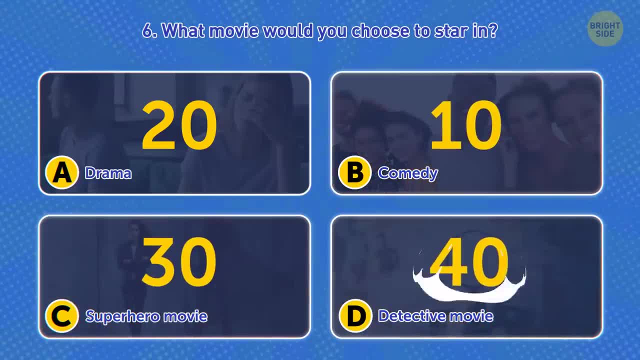 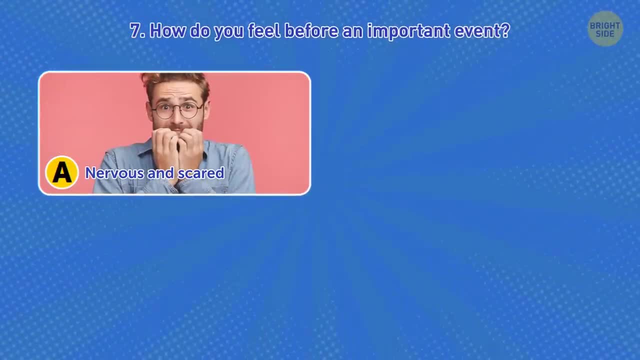 C Brings you 30 points And D Is worth 40 points. How do you feel before an important event? A- Nervous and scared. I don't want to let anyone down. B- Excited: I love to test myself and triumph. 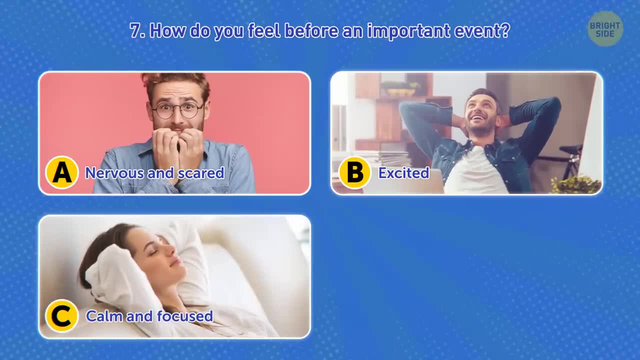 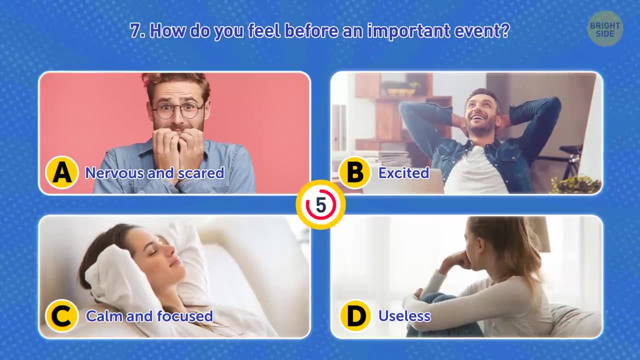 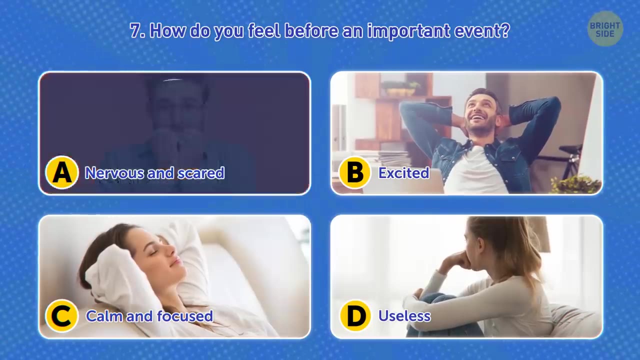 C: Calm and focused. That's what helps me always win D Useless. I always feel like others are putting more in it. If option A is your choice, you get 10 points. Would you rather go with B? 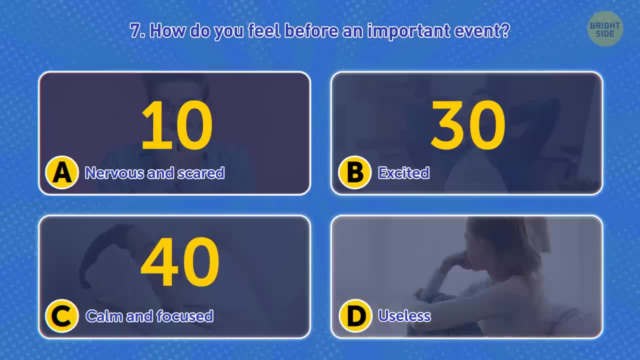 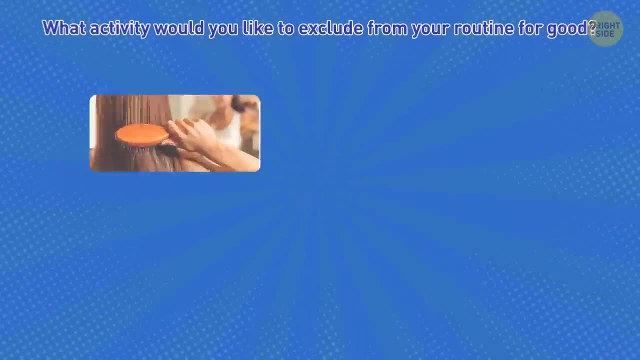 It's worth 30 points. C Brings you 40 points. D Is worth 20 points. What activity would you like to exclude from your routine for good? A? Washing, drying and brushing my hair. It's a waste of time. 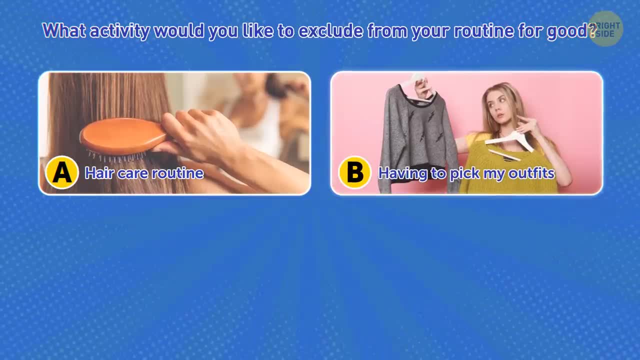 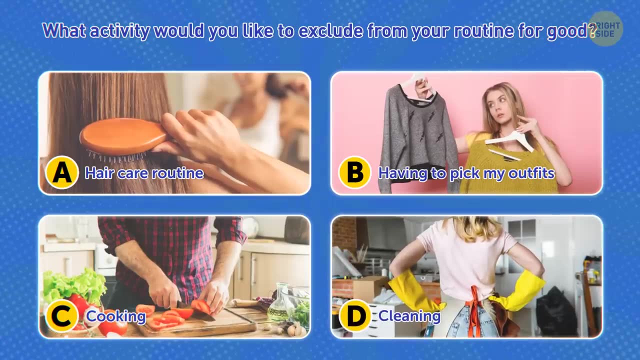 B- Having to pick my outfits: Let a robot do it for me. C- Cooking: It's definitely not my thing. D- Cleaning: Things turn into a mess again too soon. If option A sounds like the way to go, give yourself 10 points. 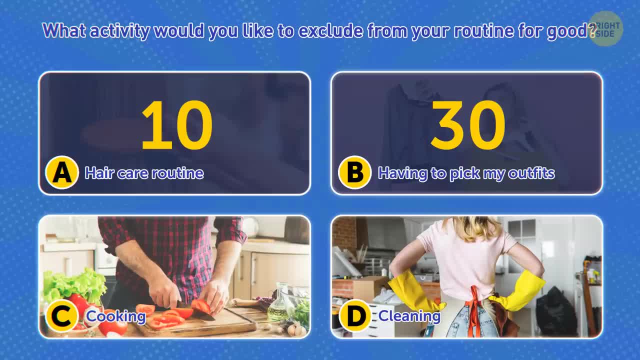 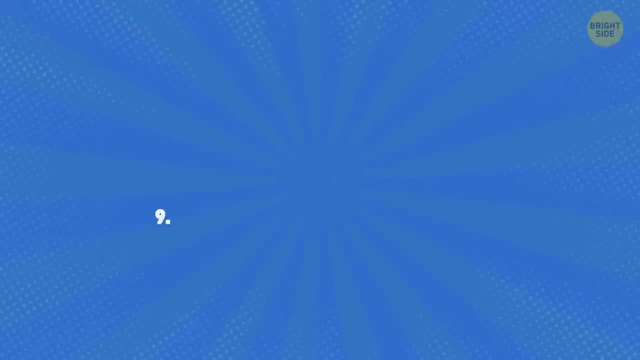 If B is your choice, you just scored 30 points. In case you went with C, add 40 points to your basket. Finally, D brings you 20 points. Which sense do you rely on the most? A Smell. 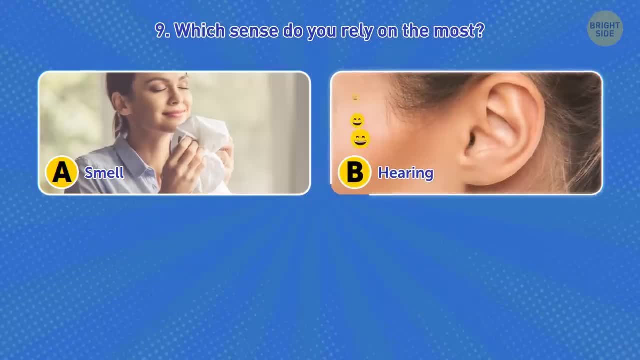 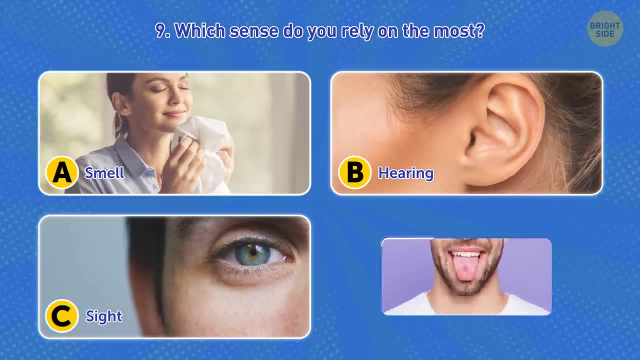 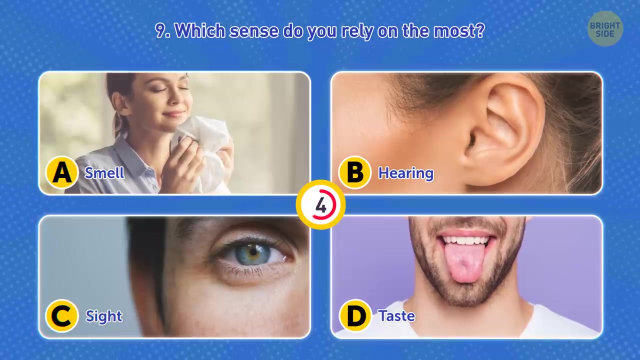 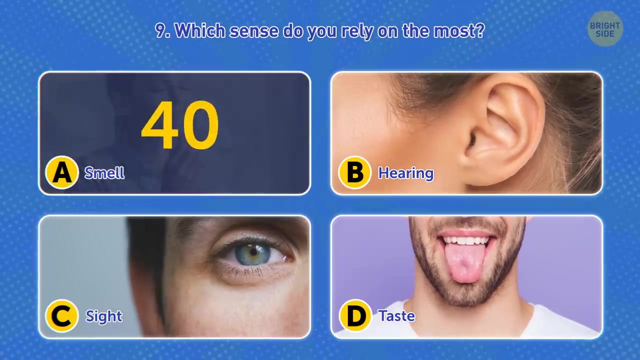 I could create my own perfumes. B Hearing: I can hear someone whisper across the street. C Sight- They say I have eyes on my back. D Taste- It has never let me down. If you went for sense of smell, you get 40 points. 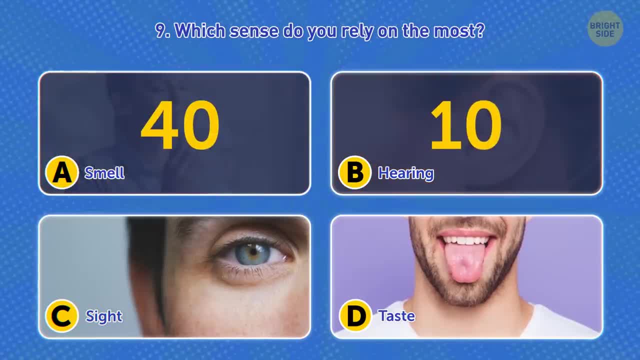 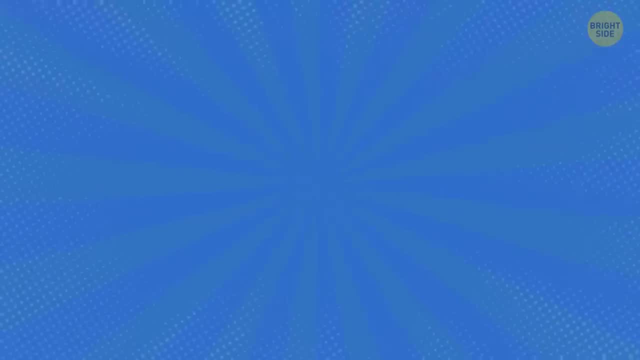 Those who trust their hearing get 10 points. If you have an eagle eye, award yourself with 20 points. Your sense of taste brings you 30 points. You're arranging a first date with someone you really like. What is it gonna be? 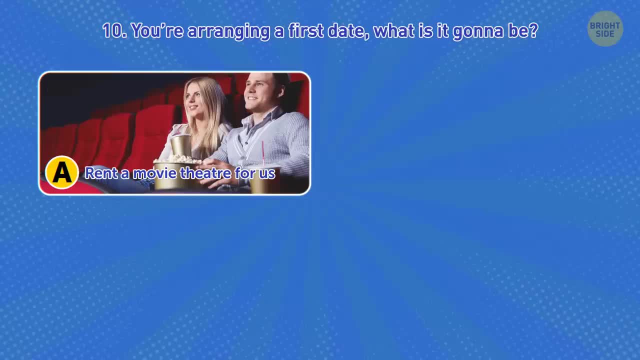 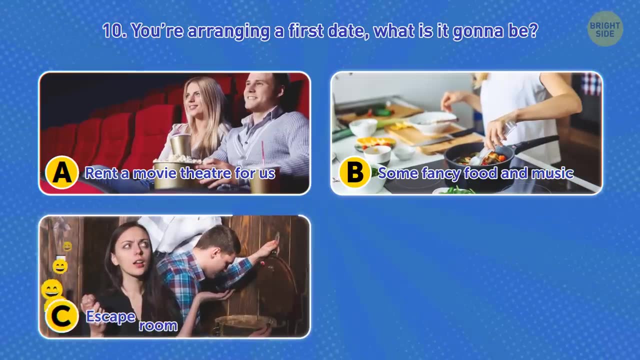 A- I'll rent a movie theater or a planetarium just for the two of us. B- I'll cook some fancy food and learn to play some musical instrument. C- I'll take them to an escape room and let them show how smart and brave they are. 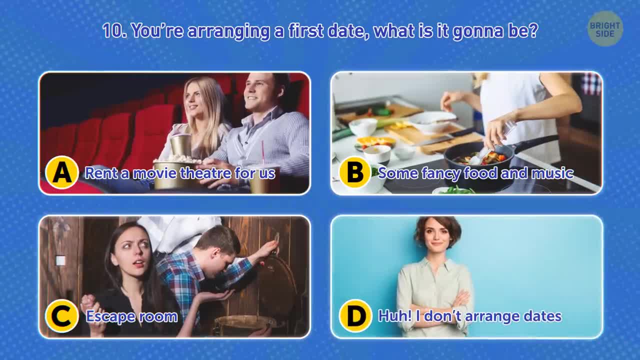 D. Huh, I don't arrange dates. Others try their best to impress me. I'll take them to an escape room and let them show how smart and brave they are. Others try their best to impress me. Option A brings you 10 points. 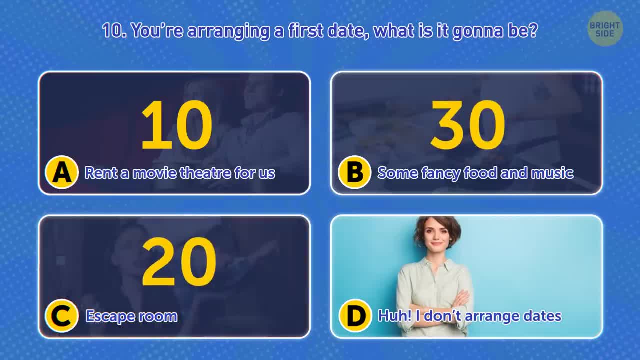 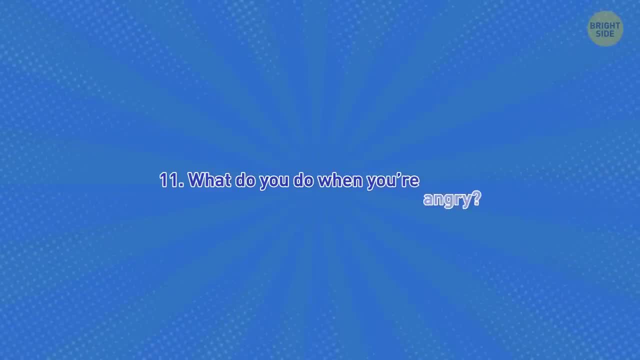 B gives you 30 points. Option C is worth 20 points. If you chose option D, here are your 40 points. What do you do when you're angry? A Ignore everything and everyone. I need some time to cool down. 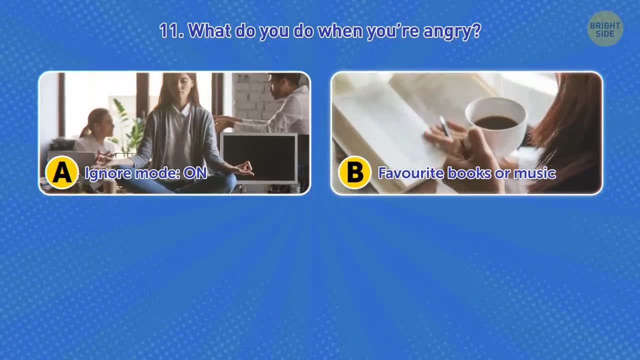 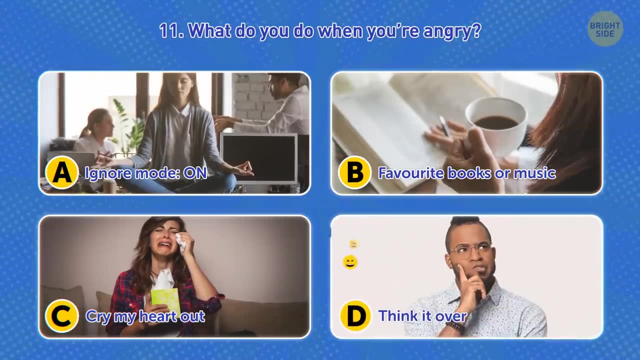 B Read my favorite book or listen to something. C Play some music. C Cry my heart out. It helps me restart my system. D Think it over. I gotta understand what made me so angry and how to avoid it. 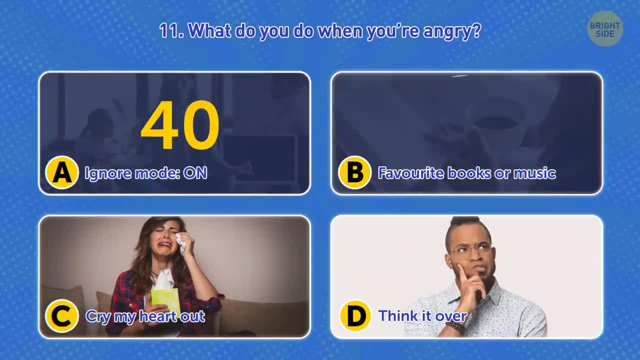 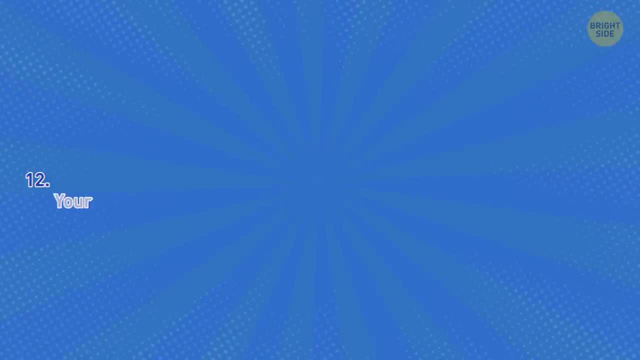 Option A adds 40 points to your basket. Option B gives you 30 points, C is worth 10 points And D is worth 20 points. And D is worth 20 points And D is worth 20 points. Your friend's having a housewarming party. 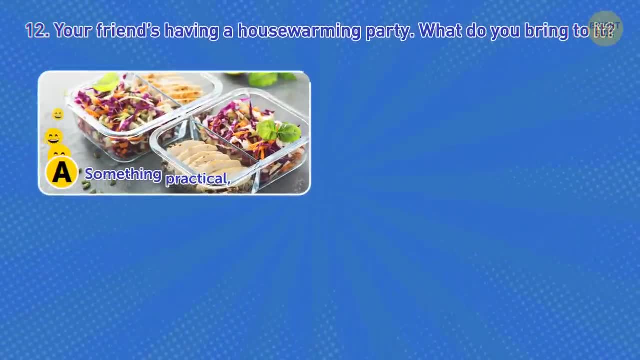 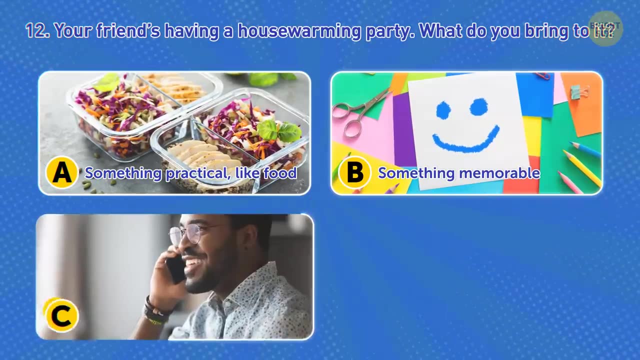 What do you bring to it? A- Some food or something else practical will do. B- I'll write a poem or make a fun collage and frame it to make it memorable. C- I'll just ask them what they need for the new house. 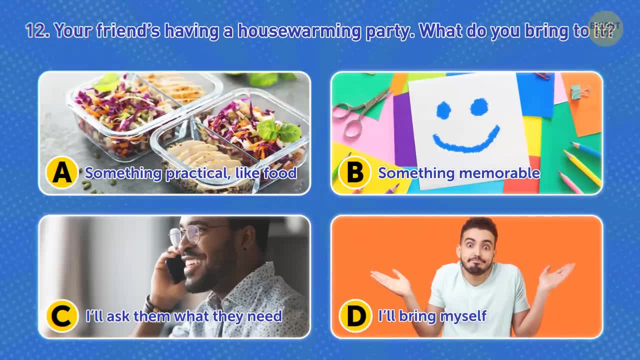 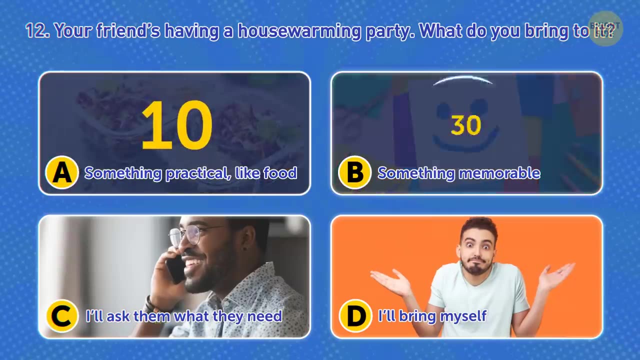 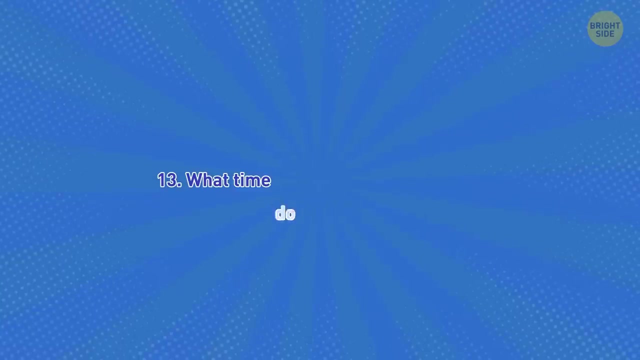 D, Hmm, Nothing. My presence is the best gift. In case you chose option A, give yourself 10 points. B adds 30 points to your score. C is worth 20.. And D is a 40-point option. What time do you usually go to bed? 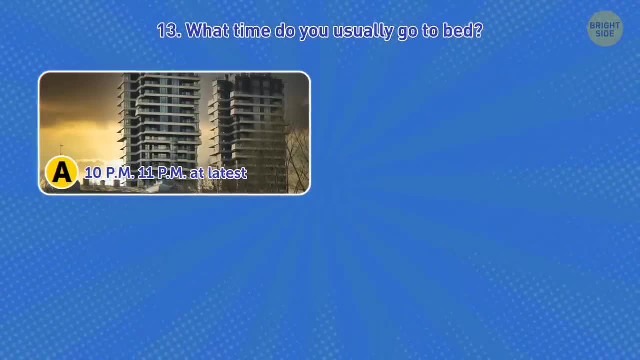 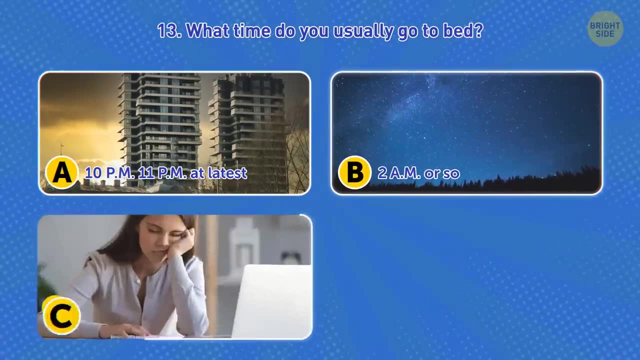 A- 10 pm, 11 pm at latest. I keep it healthy B 2 am or so, And then I wake up around 2 pm. C- What is sleep? I never get any. 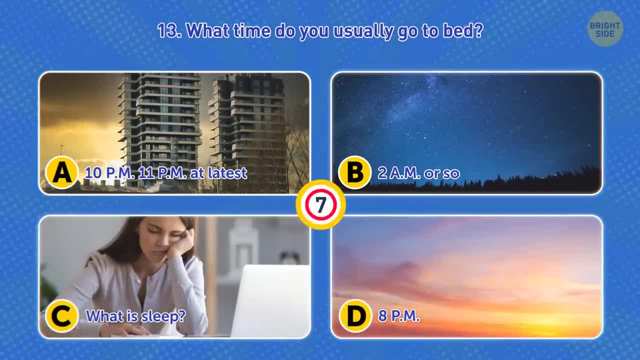 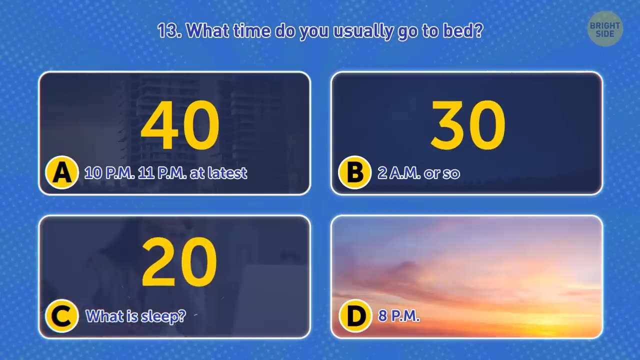 D: 8 pm. I need my beauty sleep. A- 10 pm, I need my beauty sleep, I like it. Healthy sleepers get 40 points, Night owls get 30 points. Those who never sleep win 20 points. 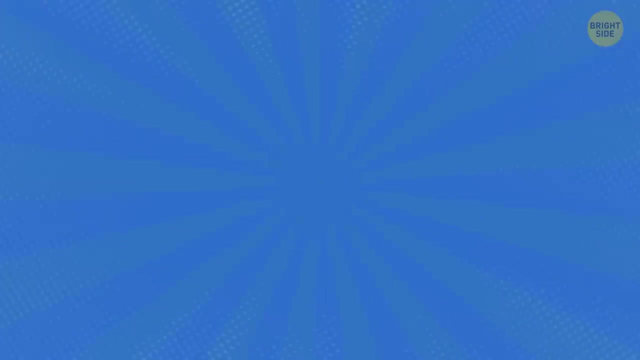 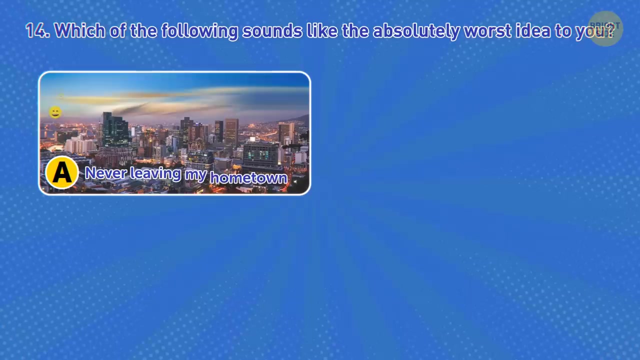 Those who go to bed early get 10 points. Which of the following sounds like the absolute worst idea to you? A- Never leaving my hometown for the rest of my life. B- Doing all the work and watching others get promoted. C. 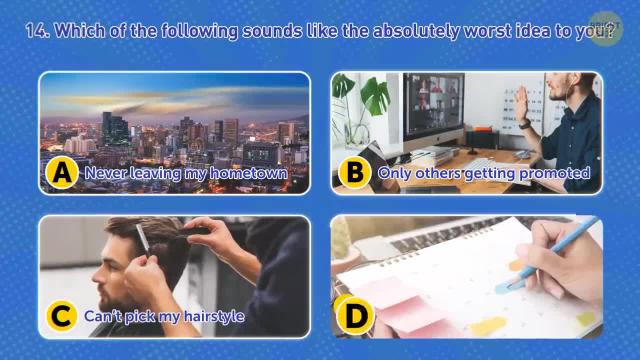 Have someone else pick my hairstyle for me. D- Never knowing my schedule, I can't live without a good plan. Those who went with option A get 30 points. Option B is worth 40 points. C brings you 20 points. 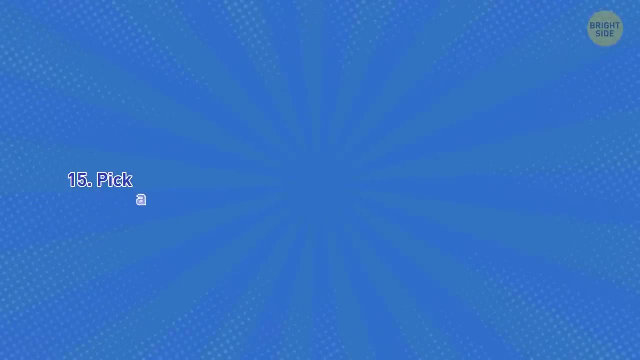 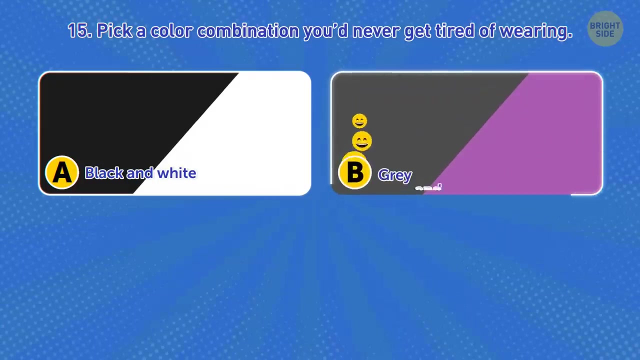 D is worth 10 points. Pick a color combination. you'd never get tired of wearing A Black and white. I'm classy. B- Gray and pink, Official with a playful twist. C- Orange, purple, emerald With a sprinkle of blue. I dress brightly.